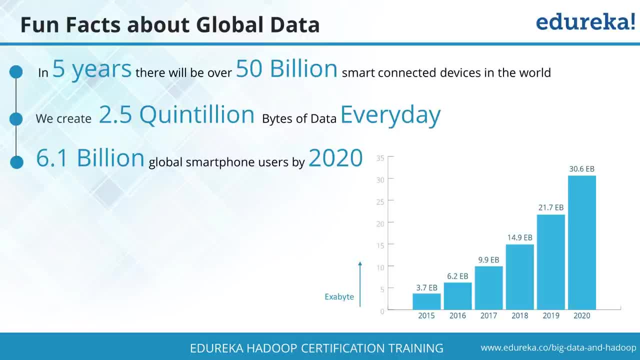 in a disk and you will be able to reach moon- twice That much amount of data we have in current world. So you can imagine when today, we have this much amount of data and that data itself we are calling that, it's very difficult to manage right now. 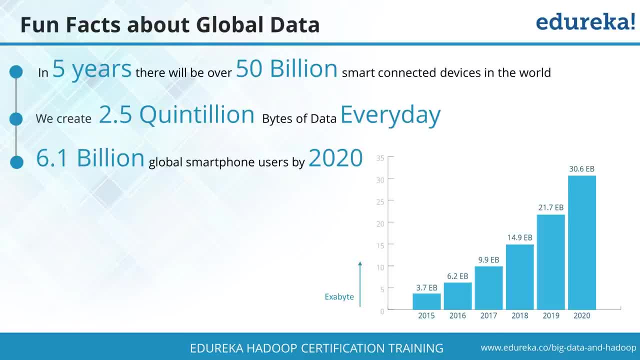 Imagine what is going to happen in 2020.. We are talking about almost three to four years ahead of the time. What is going to happen? The data will be like four times to 10 times larger what we currently have, And that is going to be a very tricky task. 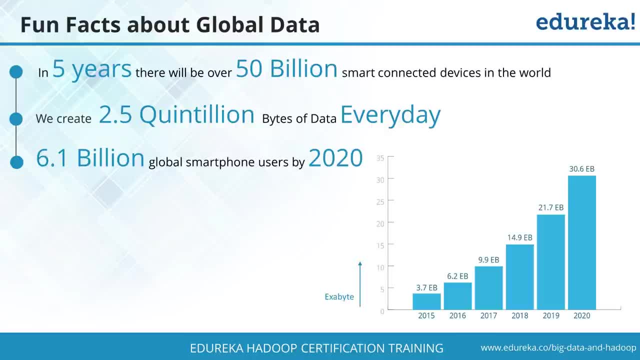 and that is where this big data tools will be very, very important. In fact, right now, The situation is that very less companies have identified the potential of this big data. Lot of companies are hesitant towards moving towards big data tools. I would say only 5% of the companies have realized. 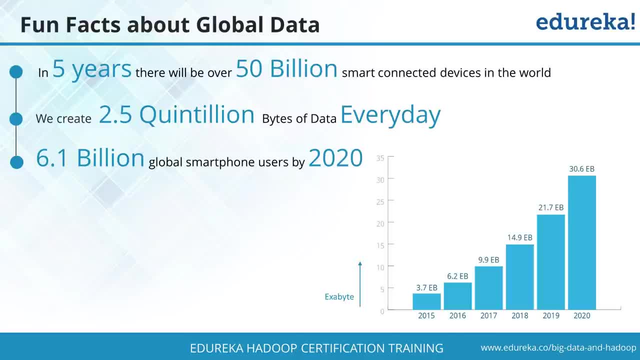 the potential of big data, And I'm only considering the companies who are like into data domain, who are dealing with this data domain part Now. among those, only 5% have realized the potential of big data And that understood the importance of big data. 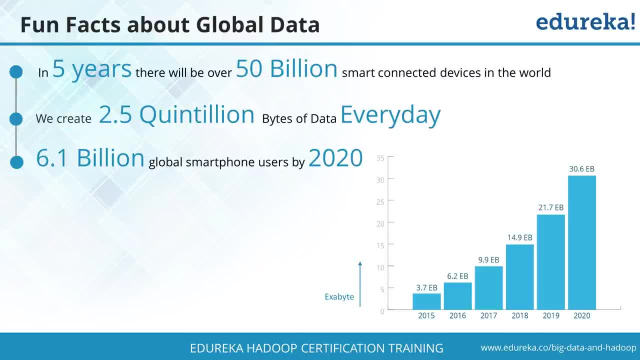 And the reason is that it's very simple. They're kind of worried that if you move from our traditional systems to this HDFS or Hadoop system, will we get people? Are there people available who will solve the problem for us? Will it be easy transition for us? 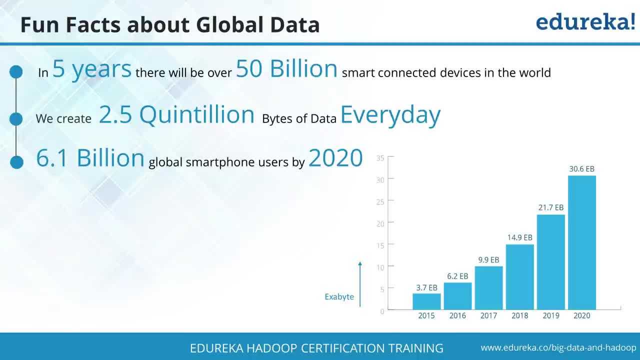 So all these, because of all these things, they're hesitant to move. But in future you are going to notice that it is going to be solved. So this is pretty sure that this problem will be solved in coming time. It will not be there for a longer period. 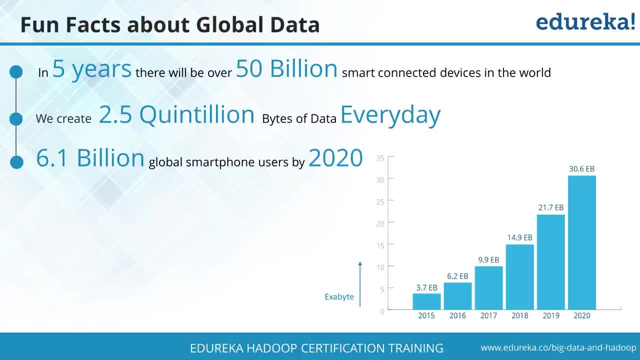 So this will be all solved, But by 2020, analysts have predicted that this 5% will get to 40%, and when this 40% will explode, you can imagine. not only data is exploding, but also job will be exploding in this domain. 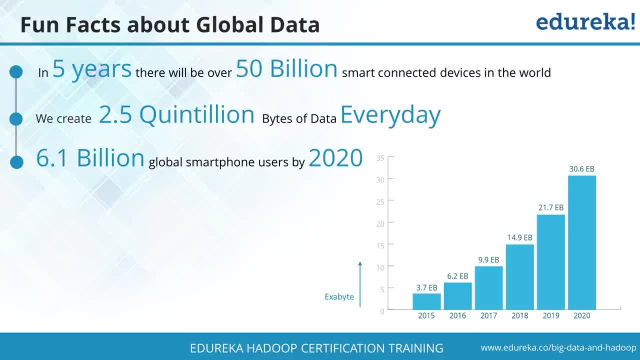 Currently, in today's world itself, we have so many jobs available. Imagine the situation in 2020.. That is going to be very interesting to look at, So let's move further. Now if talk more about the data. I just answered this part. 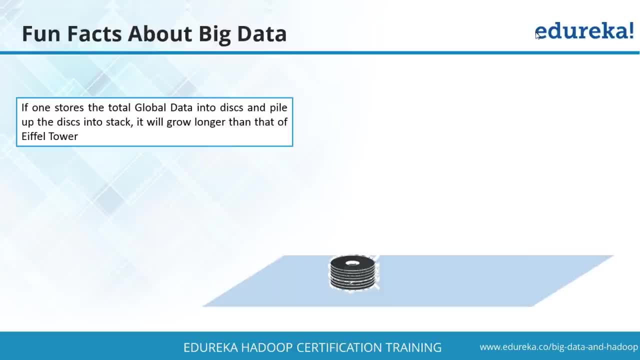 Now, if you keep on stacking it, I told you, you can reach two times the mood. Same story they mentioned about the Elphill Tower as well. So it is two huge data to talk about which we currently have Now moving further. Now, if we see this example, you can notice: 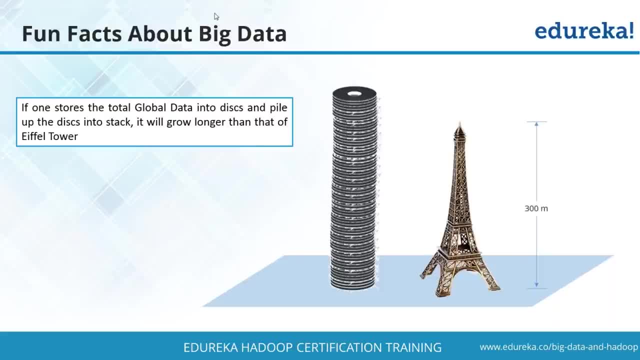 Like with Elphill Tower, the data is growing so huge that you can keep storing the data, and it can reach till the height of your Elphill Tower. That's very interesting. Now let's see what you understand by this word big data. now 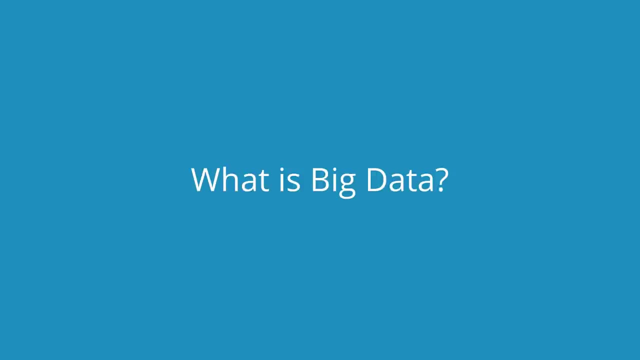 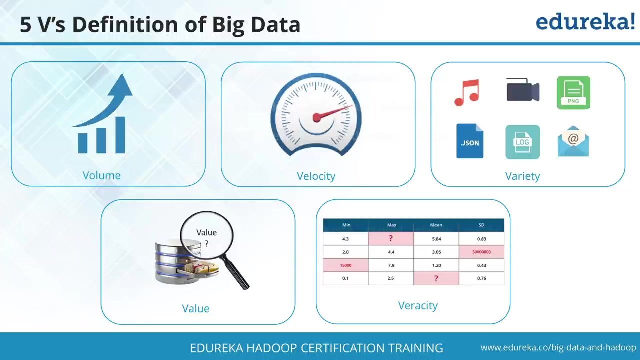 So we have just talked about few fun fact about it: that what is this? but what is big data? What do you understand by this keyword big data? Now, lot of people generally say that when I have large volume of data, I will be calling it as big data. 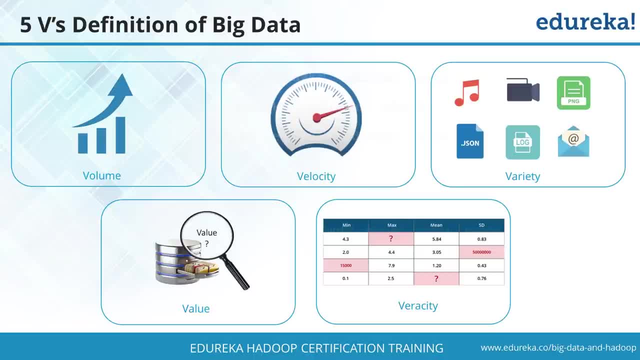 But that's a wrong notation. This volume is just one property of big data. We cannot say that if it is huge volume, then only it is a big data, otherwise it's not a big data. No, volume is one characteristic of big data. There are other characteristics as well. 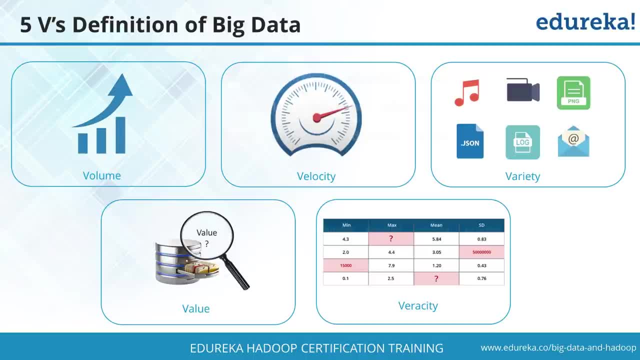 For example, now the velocity, Because if you see this Facebook, it is just 12 year old company. It is not a very old company, but currently the situation is that within 12 years they have generated a massive amount of data. Few months back there was a fun fact. 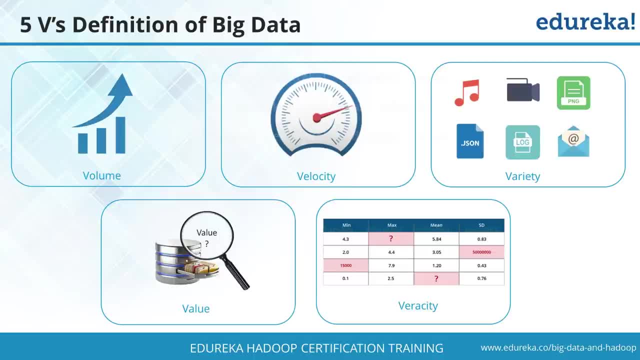 what was posted by Mark, who is the CEO of Facebook. He posted that today, the number of users who are using Facebook is equivalent to number of people living on this earth 100 years ago. That's a big statement from the CEO of Facebook. That means he is not just talking about one country. 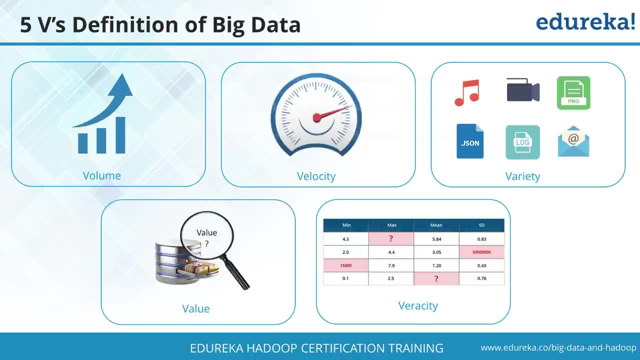 He's talking about the whole globe. Now, what does this mean? That Facebook is dealing with big volume of number of users. Now, this itself, we are just talking about number of users. right now, we are not still talked about what kind of activities or what kind of data these users generate. 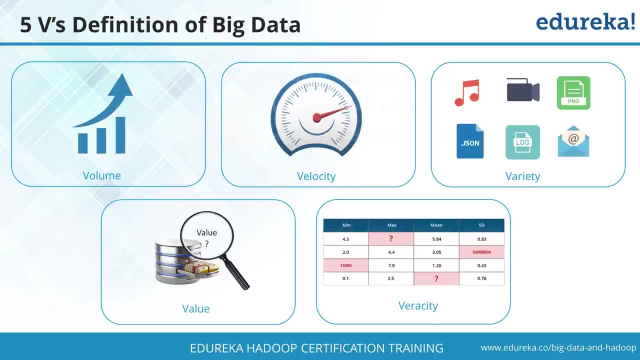 Now, if I talk about kind of data, what these users generate, we see that what we do generally on Facebook, we either put some post, we post video, we post audio, right, So we do all this stuff Now when you post video or when you post audio. 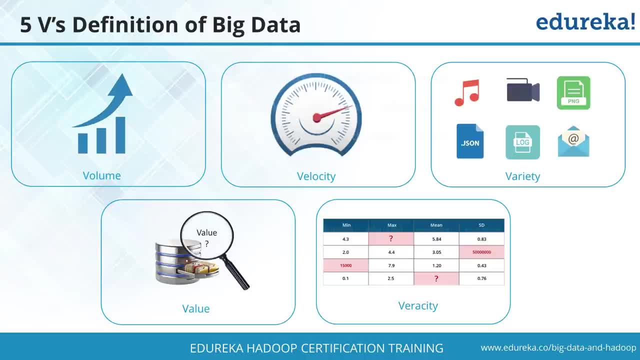 is that the data which can be handled by our RDBMS? No, because I don't have any pattern for this kind of data. It is a very different kind of data and this category we call it as unstructured data. Now, this unstructured data is a different variety. 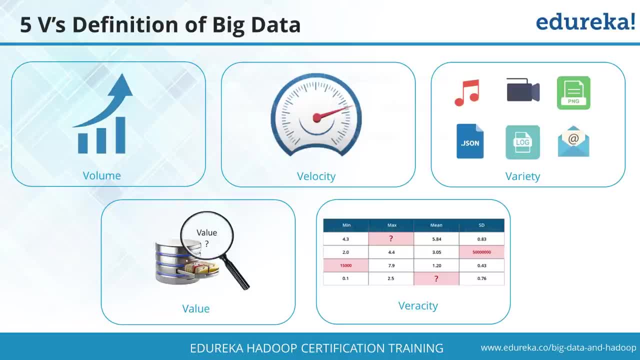 and this is growing exponentially. It is growing with a very huge pace. Now, not only this, unstructured data, even structured data also- is growing at a very huge pace, but with, if I compare both, unstructured is growing more in number. In fact, in current scenario, we have 80% of unstructured data. 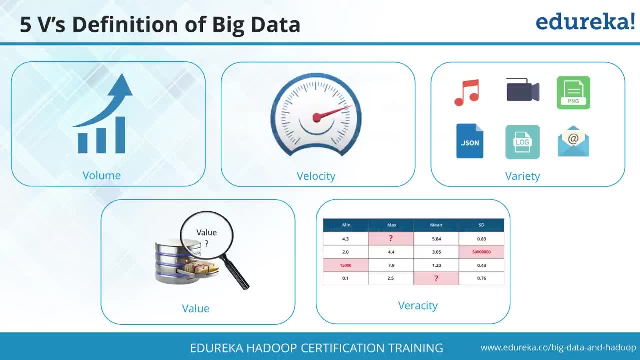 and 20% of structured data, So you can make out the importance of unstructured data in our analytics as well. Now the challenge here is that how to deal with that data. Can my RDBMS deal with my data? Forget about volume part for some time. 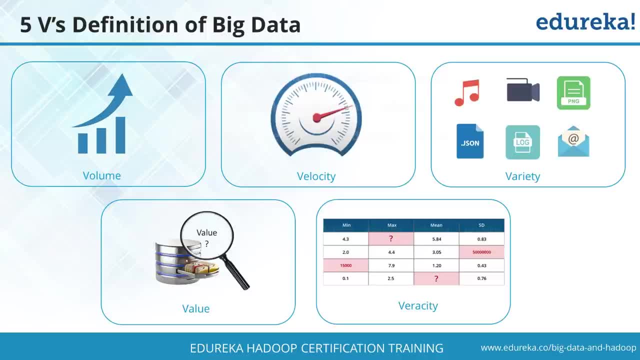 Even if it has more data. can my RDBMS deal with it? No answer will come again: a no here, and to solve this we require specialized tools like Hadoop to fix this problem Now. so that brings me to an another property: velocity. 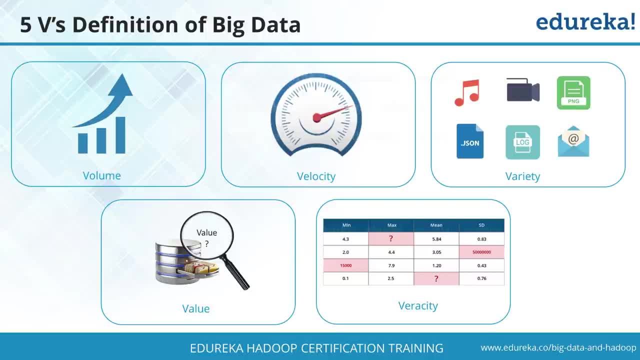 Which means the pace with which the data is growing. Also, it brings me to another step, called as variety. Like we have seen, your structured data, We have unstructured data. We are also generating data from different sources. For example, this medical domain is generating data. 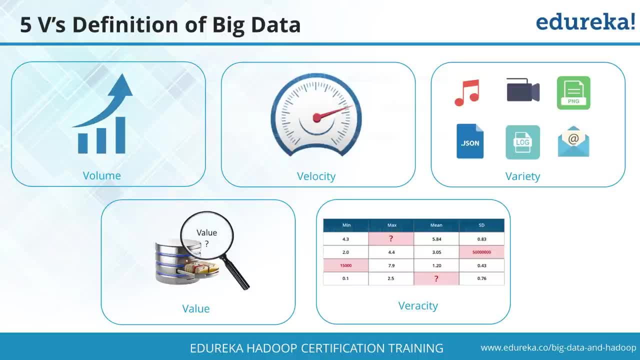 This, Facebook, social media, Twitter- all these companies are generating big data. So variety of data. what we are getting value from the data? Now it's very important. the data, what we are getting, is that meaningful data? Can I make out some insight from the data? 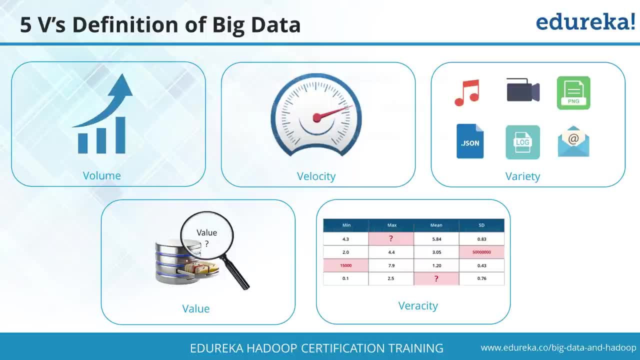 This property is called value property And the last property, which is really important property, is called veracity. In veracity, what we do is: let's say, if you're getting data, there can be data which can be corrupted, or maybe there might be data which is missing data as well. 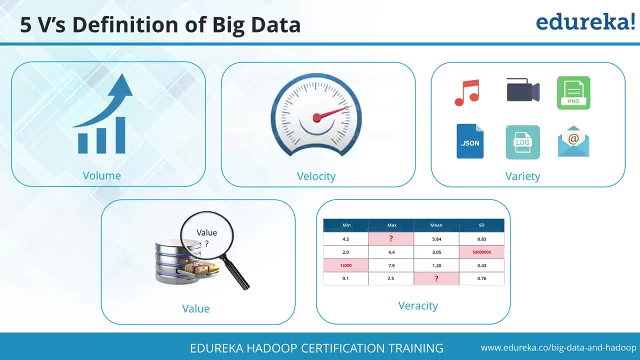 Now that sort of data where we are missing data or where we have corrupt data- how we can deal with such things. This is called veracity. So these are the five important components of big data. So we can never say just a volume is denoted as big data. 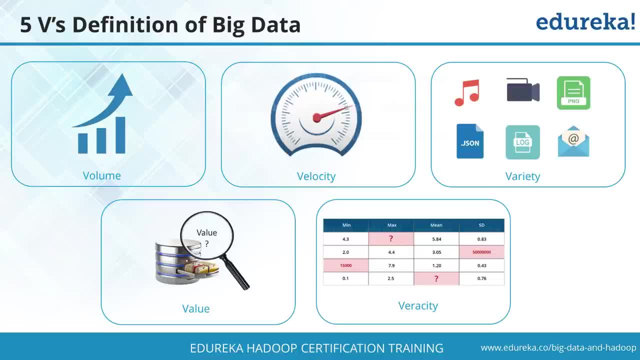 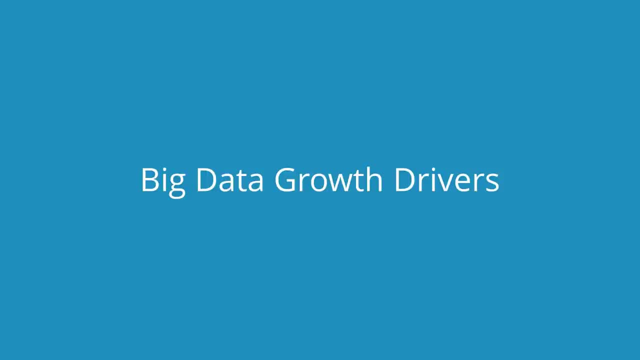 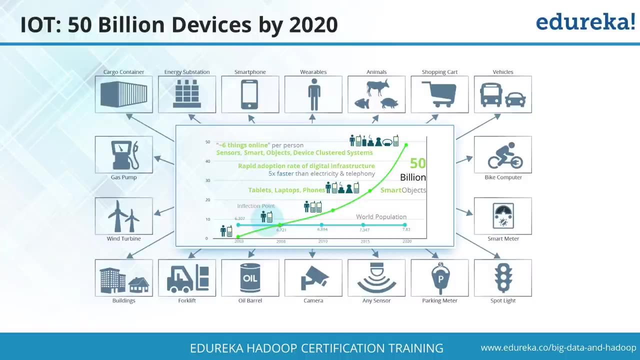 That is just one of the characteristics. There are other characteristics which are equally important. Moving further Now, data, big data, growth drives And, as we have just discussed that, imagine what would be the scenario in 2020.. In 2020, we will be dealing with almost 50 billion. 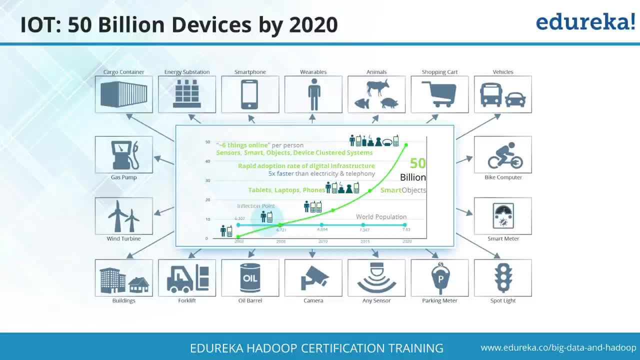 of the devices, right, That will be very huge number. We talk about any domain. we will be having such huge amount of data, So we will be dealing with so much amount of data. You might have heard about internet of devices. That doesn't going to be the next big thing. 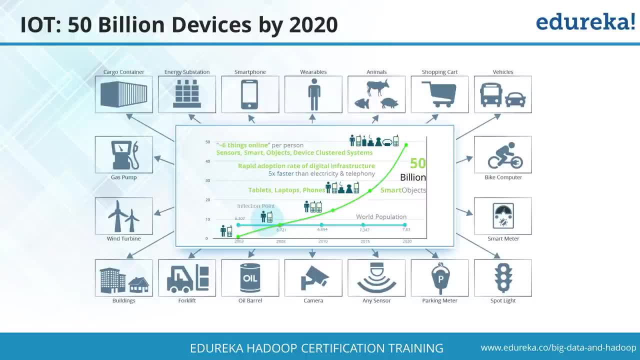 But that internet of devices is now the creating so much of huge data. right, Because here you talk about that, you can automate your home. Now there are all the devices are generating sensors. Lot of events will happen with IOT that will be all requiring big data. 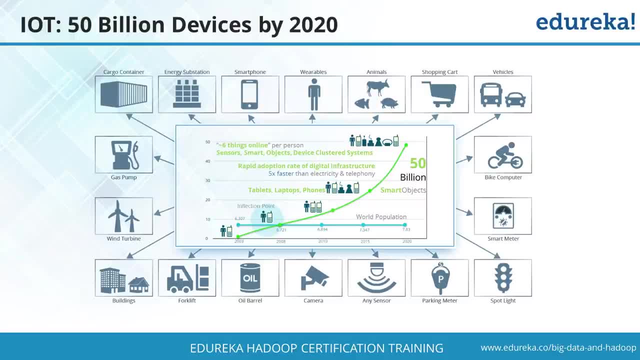 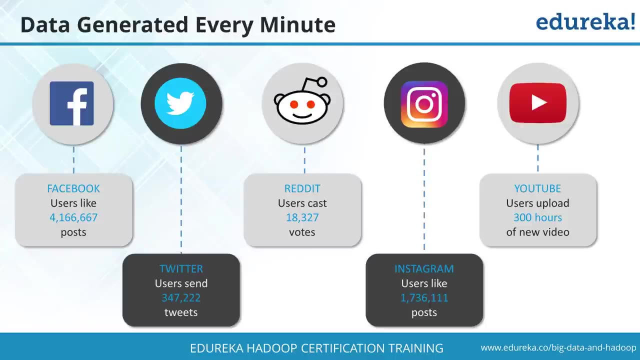 So with IOT becoming more and more popular, requirement of big data tools become more important as well. So by 2020, you can see that there will be a huge requirement of this tools to solve the problems now, every minute. I'm not talking about every day, I'm not. 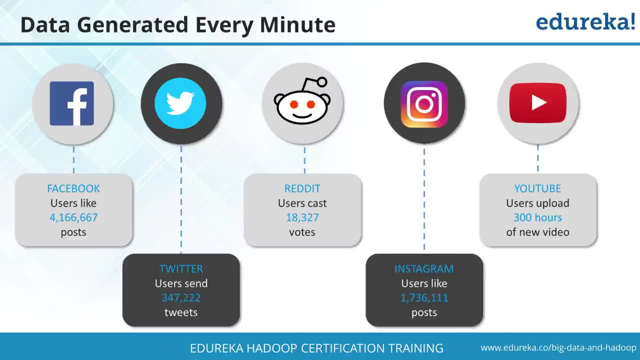 talking about every month what happens. I'm just talking about every minute, every minute. on Facebook there are so many of likes happening right every minute. we are getting almost like around 42 lakhs like we can talk about Twitter. almost 3.5 lakhs tweets happens per minute. you can even talking about others. 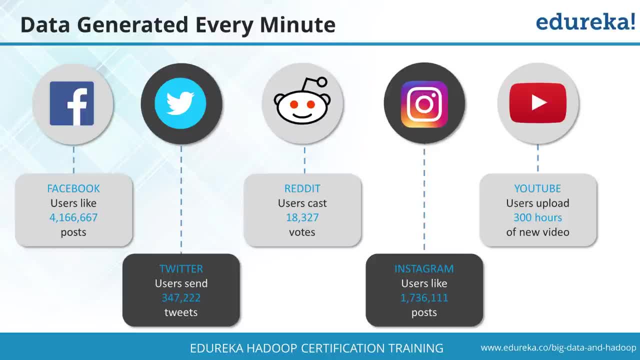 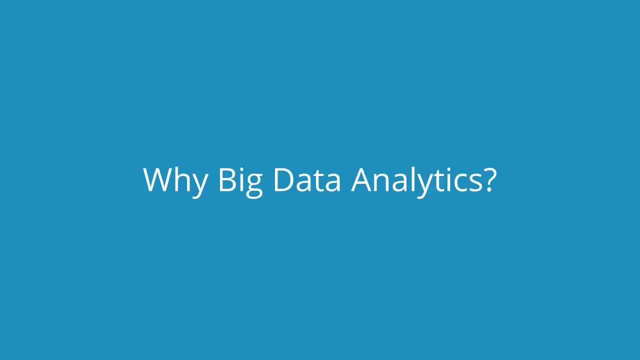 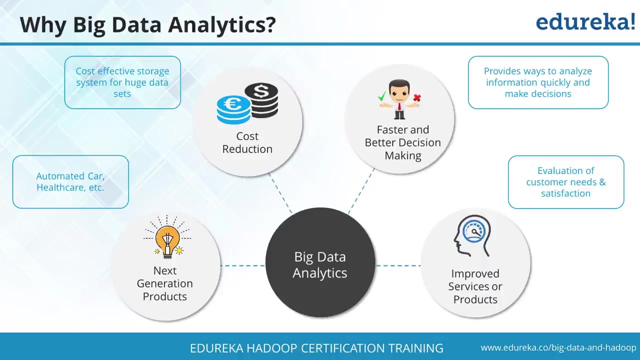 like YouTube, reddit, Instagram, like YouTube. on YouTube, almost 300 hours of data is getting generated and that is again a big thing, right? because so much of data we are generating per minute. why this big data analytics? why it is important now, when we talk about big data analytics, we have just talked about the volume which we are facing right now, but can we? 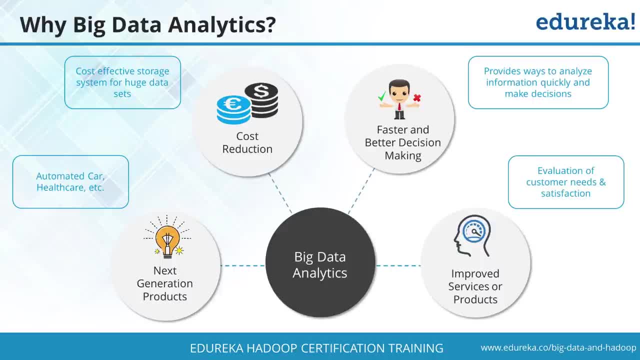 make some insights from that data. right, that is big data analytics. but why? why this is important for us, very important part: when we analyze something important from our data, maybe we can gain some business insight. so it is going to make your system cost effective. so we are going to. 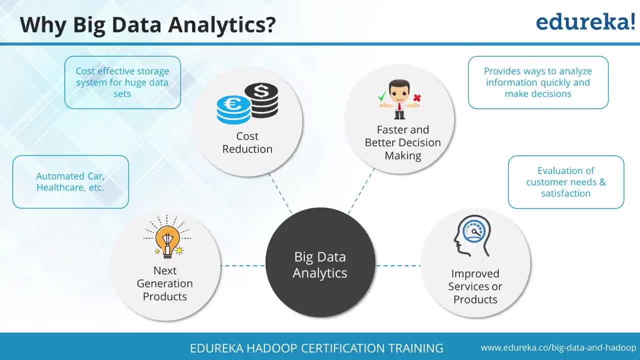 reduce the cost by analyzing it. maybe we can analyze something, we implement something in a way that it is going to save us a good amount of cost. you can also automate a car, right? so let's say, we talk about google. they have the self-automated cars and all how they did all that you might have. 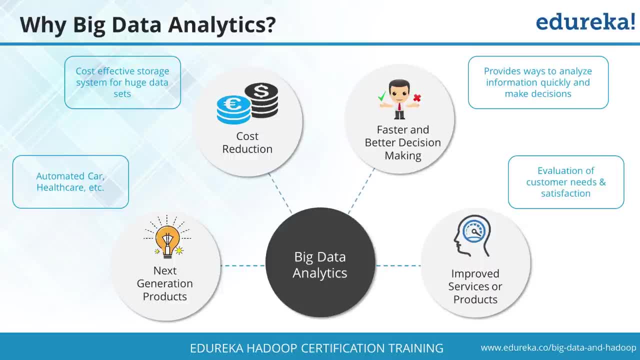 heard that they are using artificial intelligence and machine learning a lot. now these all are part of the analytics now big. they are generating huge amount of data and they are performing all sort of analytics. so this google self-driving car is the best example for this big data analytics as well. similarly, in healthcare, they keep on devising. 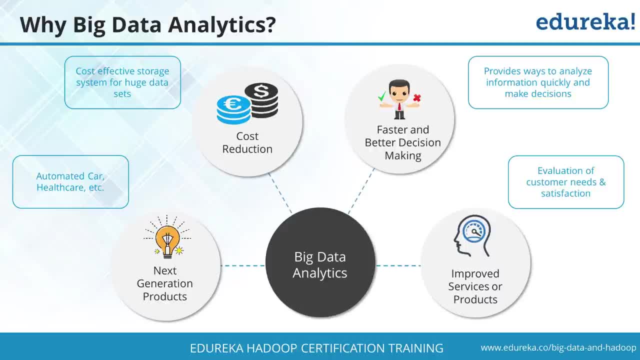 all this instrument because they have such a huge amount of data. they make some analysis on top of that and try to get some insight from it. similarly, you will be able to make the very fast decisions and those decisions will be very fast and you will be able to make the very fast decisions. 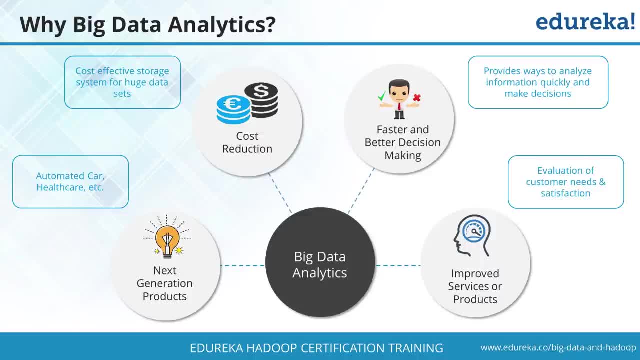 very much helpful for you. you can also improve your services for your product by analyzing the data. let's say your users are giving you a lot of reviews. now from that reviews itself, you should be able to make out some insight. that, okay, looks like there's a trend in my negative reviews. 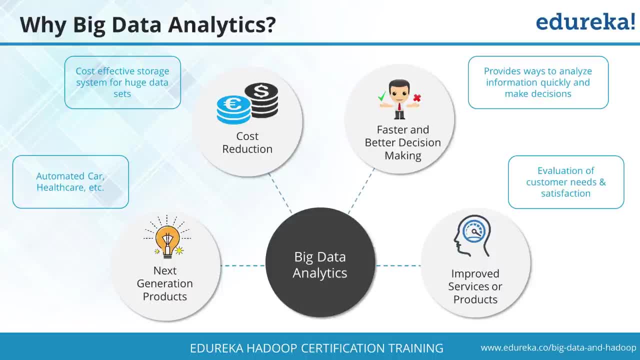 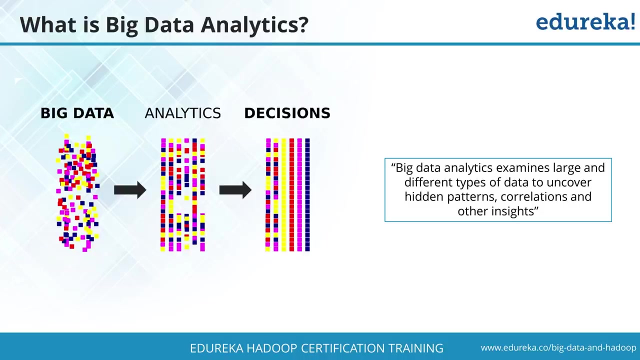 if I fit that, actually I can make all those negative reviews to positive reviews, so all those analysis can be done by big data analytics. so this is the very kind of important part and that is the reason we require this and that is the reason you are hearing from lot of companies about this job. what is big data analytics in big data analytics? let's 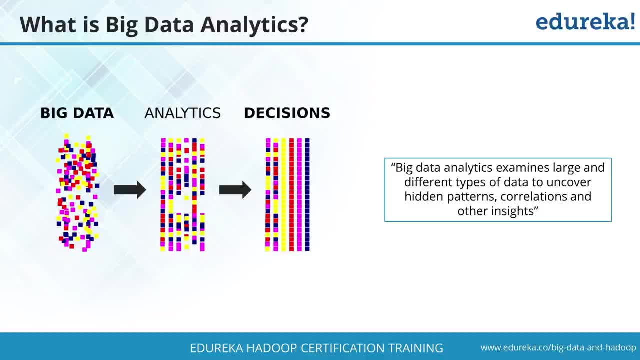 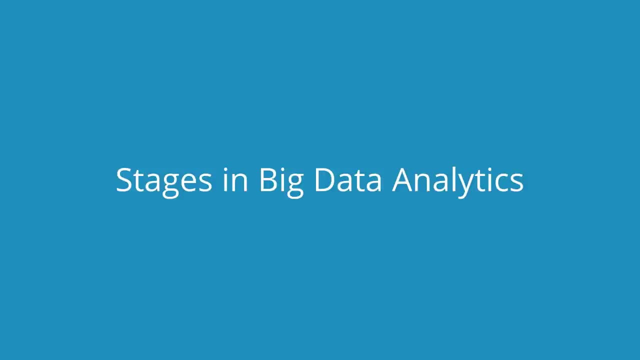 say, you will be having a big data, you will be performing your analytics on top of that and, in the end, you will be making some decisions out of it. so this will be your big data analytics. similarly, what are the stages in your big data analytics? when we talk about big data analytics? 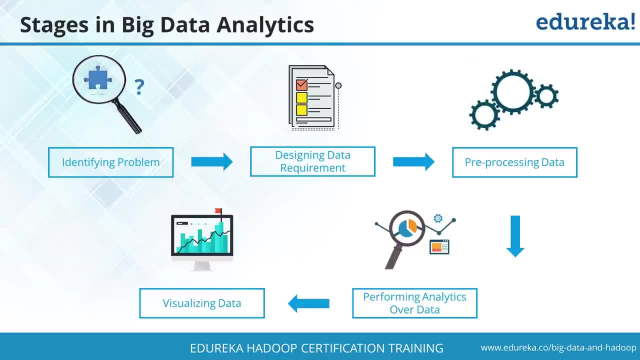 first thing would be: definitely we want to identify what is the problem we are trying to solve. What is my data requirement? that will be my second step, because first of all I need to identify the problem. then I will be add in T file the data requirement. then we will be talking about: we need to do some process and maybe we want to clean up. 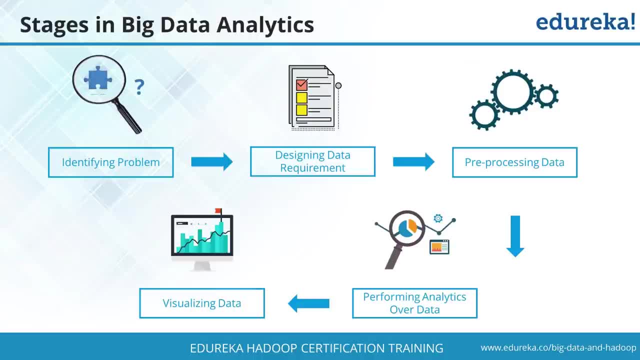 our data data. we want to do some sort of processing on the data, so that's called pre-processing data stage. after that, you will be performing some analytics on top of that. when you finish your analytics, you will be pushing it to visualize the data. that visualization can happen with 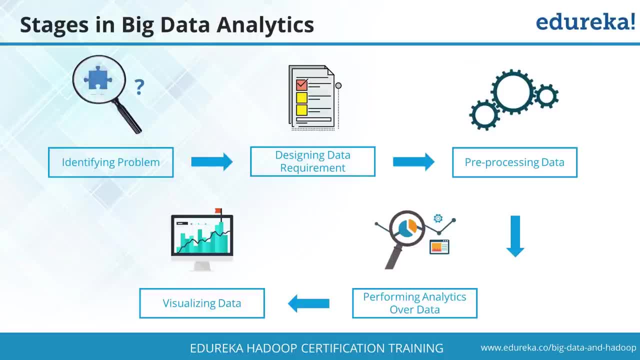 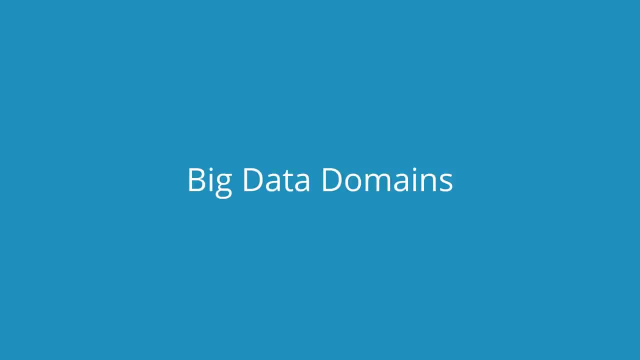 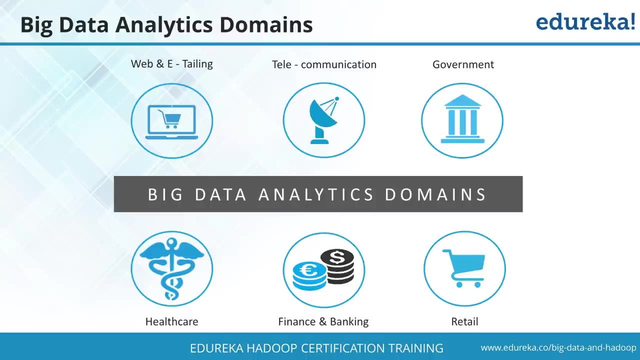 tableau, angular js or any sort of tools which are available, but you will be visualizing all your data in the end. what are our big data domains? which are data? we have web and e-tailing, for example, e-commerce, flipkart, ebay, all these companies they are analyzing. 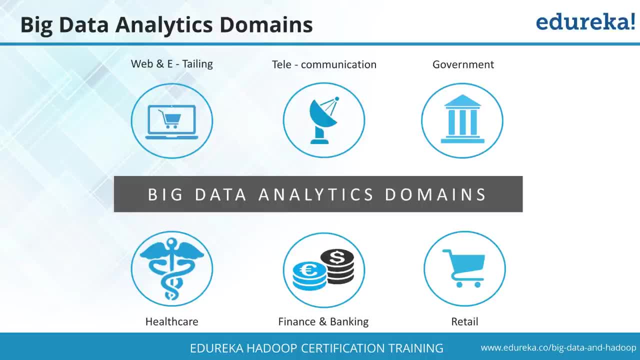 their product in order to increase their sales. telecommunication companies, companies like atl, at&t, vodafone- all these companies are using in order to perform some analytics and see That. okay, what are the customers who are at high risk of leaving us churn rate? they want to reduce that. now, all this, they do it with the help of the data, what they have available. 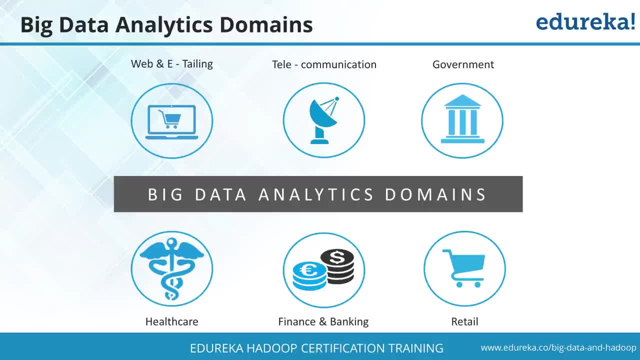 similarly government in. if you are in India, you might have heard about aadhar card. that's a very big project what Indian government has started. and now the challenge was: there are so many people living even in that aadhar card project is using Hadoop. if you just google. 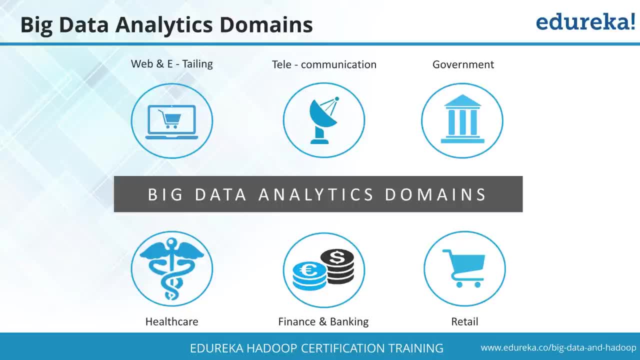 about it. you will be able to see that. Okay, you will get an idea. they are using Hadoop system in order to process them. healthcare, finance, banking- all these domains also use big data analytics. so, as you can see, these are just few list what is in front of us. there are many more fields or domains where this 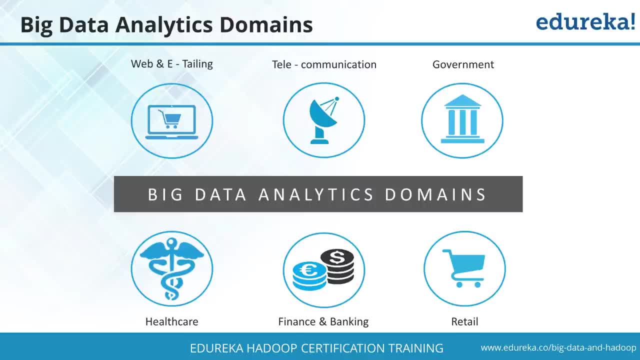 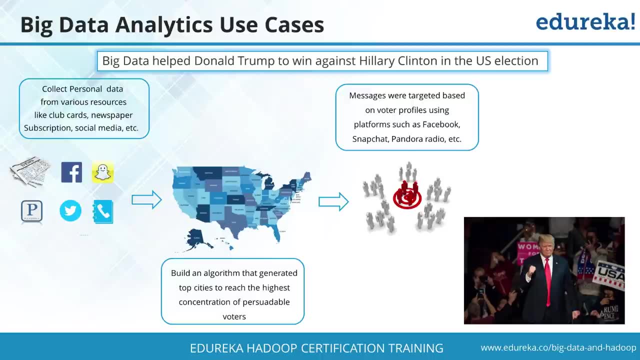 big data analytics is getting used. Now, what are the use cases? what we do have? so let's understand this. everybody must have heard about Donald Trump right, who won this US election. he is the president of US now. this guy used big data analytics and that helped him to win the election. what they did? 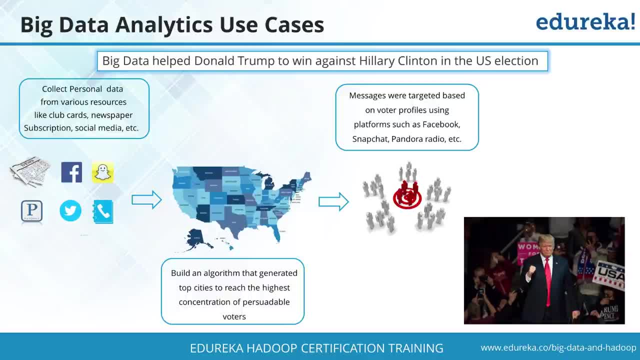 was. he collected all the personal data from various resources, whichever was possible, like club cards, newspaper subscription, social media etc. he built an algorithm, means he did not build. he had an agency Who built all that got him that generated top cities to reach the highest concentration of voters. now what he did? he kind of kept on sending some sort of advertisement or lot. 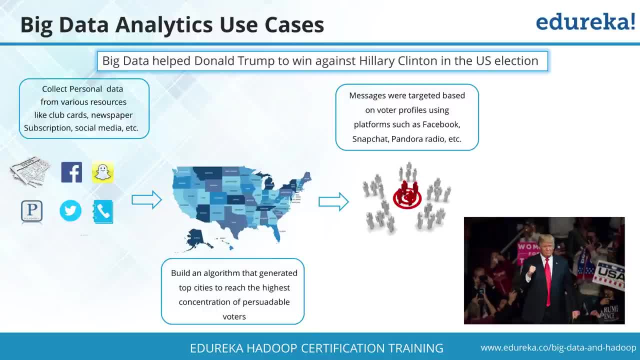 of things he kept on doing. so he first identified what are the possible voters in the domain and then, based on that, he kind of keep on publishing lot of things. and then the message were targeted based on the voter profile, Using the all the social media platform like Twitter, Facebook, Snapchat. so what he did 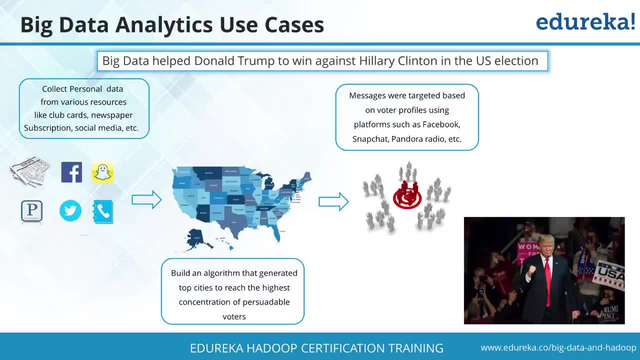 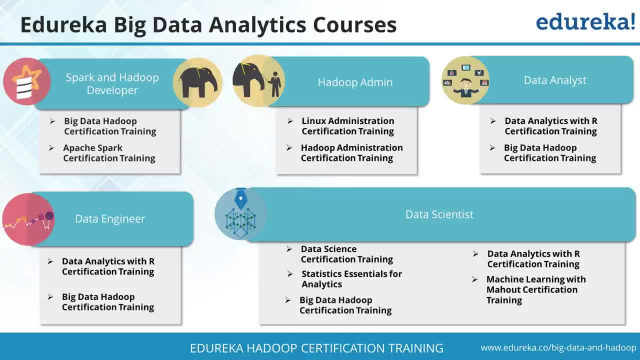 media platforms like Twitter, Facebook, Snapchat. so what he did? he kept on sending all the social like 8.30 pm to 10.30 pm ISP. they are all good after coming back to office. we have weekend sessions running as well, because a lot of people say that I am not good with. 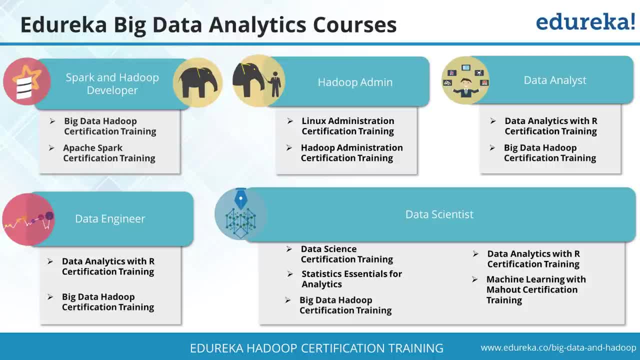 big days. I want something in weekend. so in weekend we have 8 to 11 am ISP sessions. similarly, we do have sessions in the evening as well, on weekends, which are like 8.30 to 11.30 pm. so all the times we have. you just ask the time we have it right. so even for 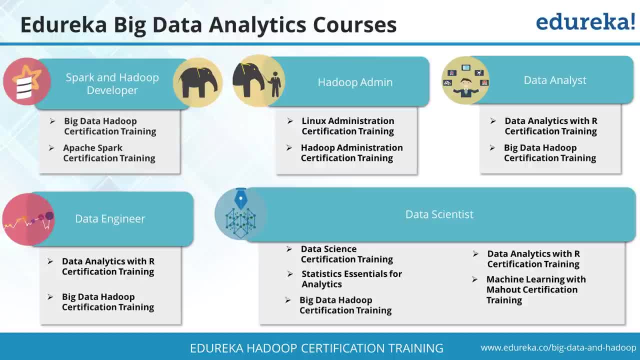 working people. we have to made the time in such a way that it should suit all the working people as well, so that's not a problem and you will be getting a good, sufficient and ample time to complete everything up question from with. I am a pressure. what would be best? 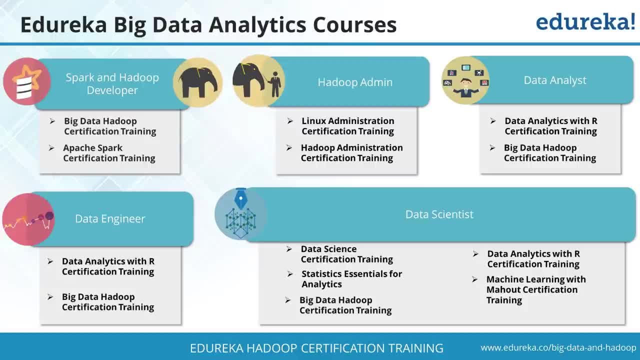 for me, my suggestion would be go for big data Hadoop developer first, followed by Apaches first. these two courses are must if you want to excel in big data analytics field. now other course are still like important, for example, this data scientist course. the reason it is: 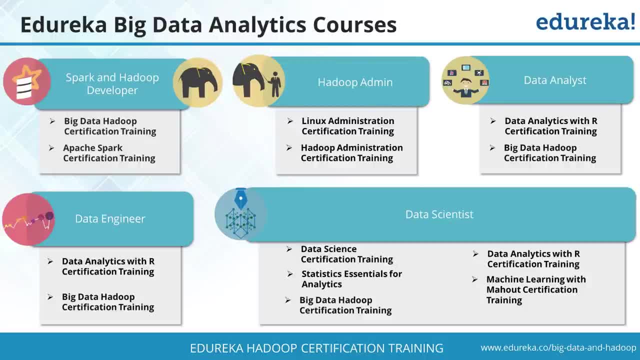 important is because you might have heard this language, R, which is majorly used by analyst. this is like a hot selling cake in the market, right? because lot of companies started using this R language. they want to now start doing analytics, and they want to start doing analytics. 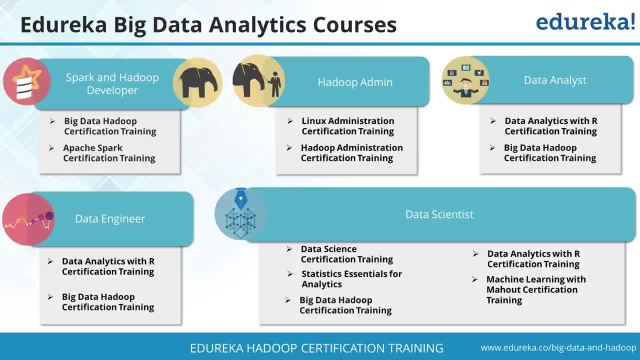 with that. so that is the reason it is the one of the hot topic in the market and lot of companies are looking for it. so definitely, this is also important. but, to start with, you should look forward towards big data Hadoop developer, followed by Apaches, and that would 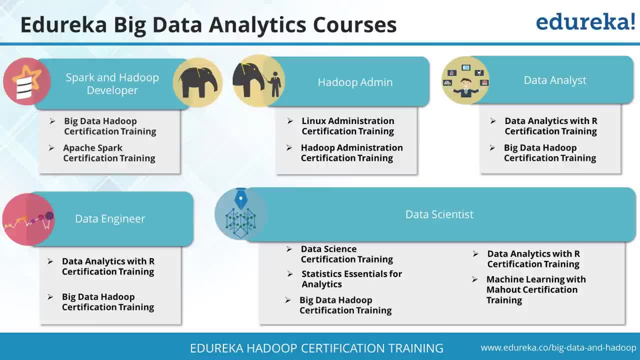 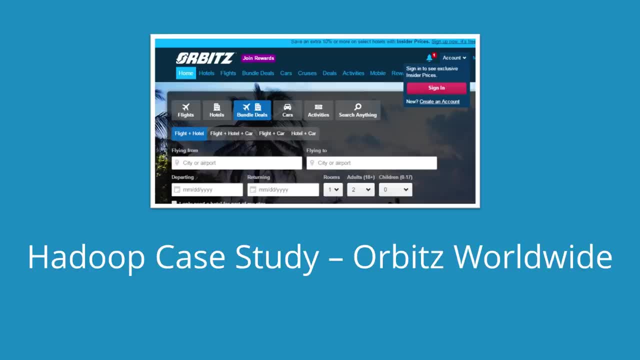 be my solution with even for you as well. whoever are experienced people, same solution will go. now let's see interesting case study. we have just talked about this Hadoop and all that analytics Part, but let's see an interesting case study. let me explain you what exactly this is. so 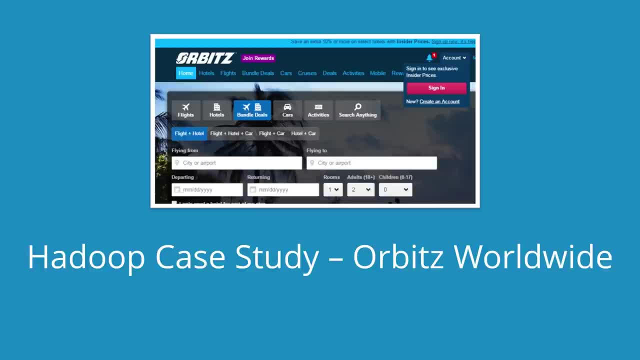 I'm not going to go deep into this topic, just to give you an overview of that: when you do all these courses, what kind of projects you will be solving. so this is just to give you a glimpse of the project part. so there was a company named as Orbitz that used to like 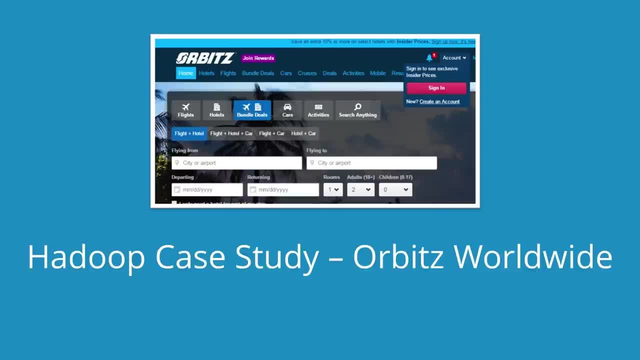 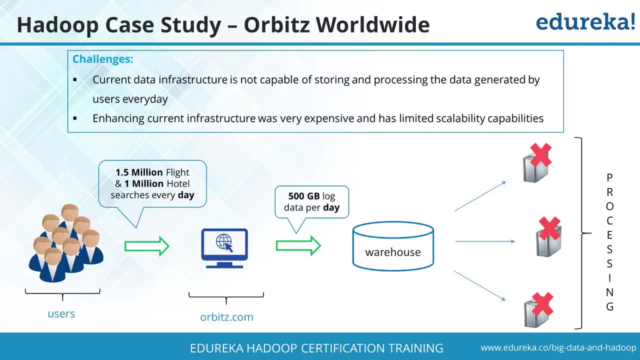 book the portals booking flights, and all that. now they were facing some issue. the issue what they were facing was: They have some challenges. the data, what they were dealing, it was huge. there was so many users coming and to their website. now they were using warehouse to solve their problem. 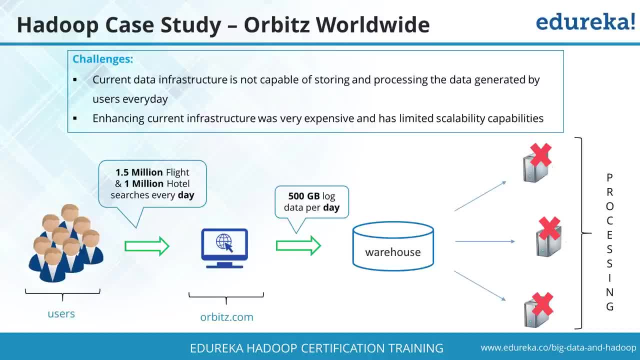 for your processing means. database is concerned enough, but with so many users, almost 1.5 million flights, 1 millionth of portals, searching each day was almost impossible, and that's the reason they were generating even 1500 GB of log data per day. 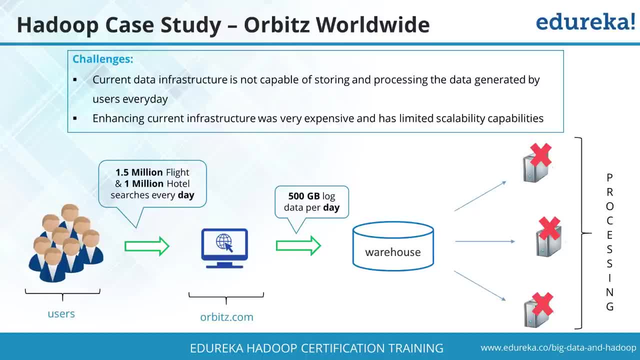 That's the reason they were generating even 1500 GB of log data per day. Now, with warehouse growing like this, it was almost impossible to process it. so this was the biggest challenge for them, and to solve this they started using Hadoop. so they were. 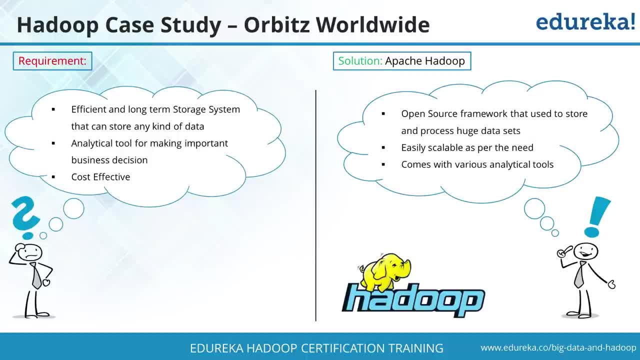 looking for all these problems. that- okay, I want something efficient and long-term storage system that can store any kind of data- means I'm not only worried about structure data. even my unstructured data should get stored. can I have some analytical tool which will help me to analyze my data, and it should also be cost-effective. 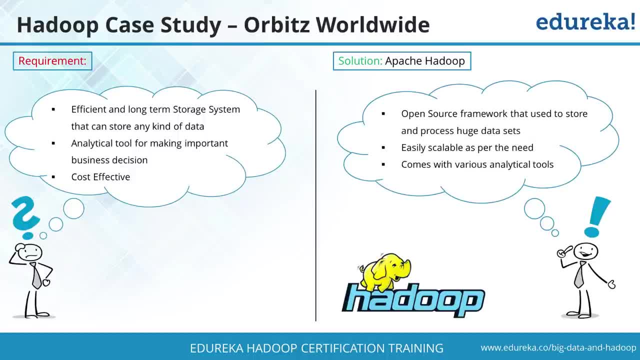 Now to get that answer. Hadoop answered it stating that, yes, I have all your answers. open source framework it is, so it is free of cost. you will not have to apply any of the costing factor here. it's very easily scalable and it has lot of analytical tools, which helps. 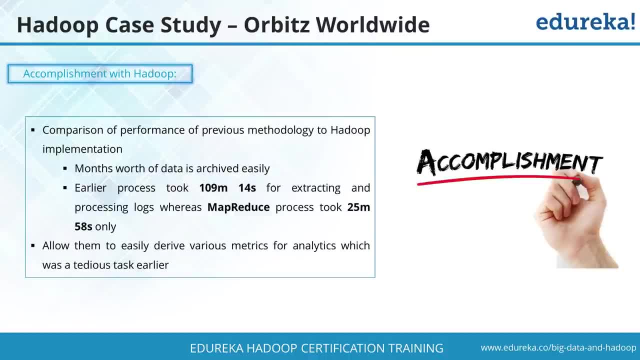 you to solve the problem. so what they did? they accomplished their solution with the help of Hadoop part. they have kind of used lot of Hadoop tools to solve the problem. they used MapReduce, they have used Hive, so these tools they were using to solve the problem. 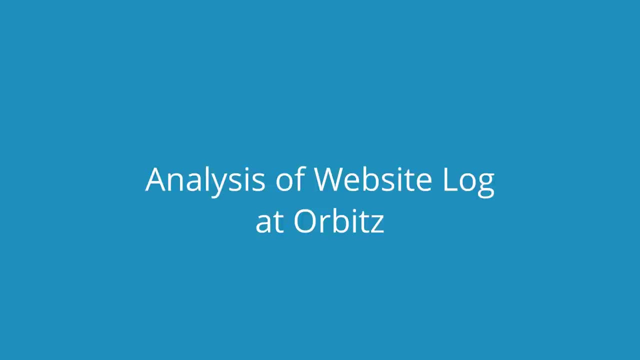 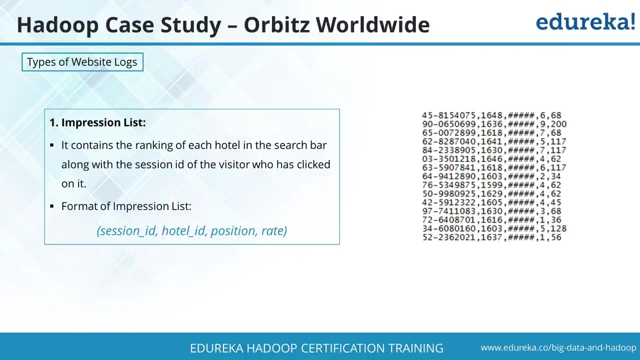 Now let's see that how the analysis is happening of website loss at Orbitz. so what they had was they have two kind of data now. the first data was impression list, where they have a session ID, portal ID, the position. the position was important. now what was happening? let's 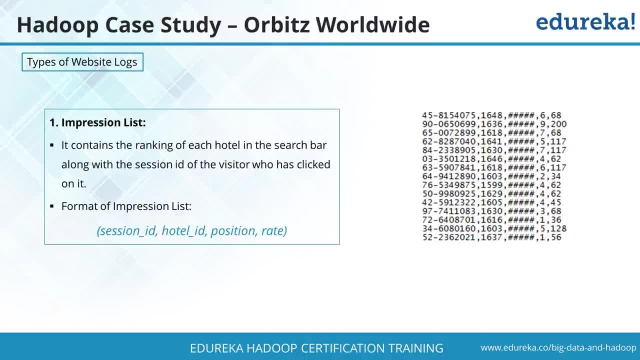 say, when you search something, it shows you a page and it shows your page of list of portal. now how it should decide that this should be my first page means in the page also itself. that should be my first link. this portal should be page that first link. this hotel should. 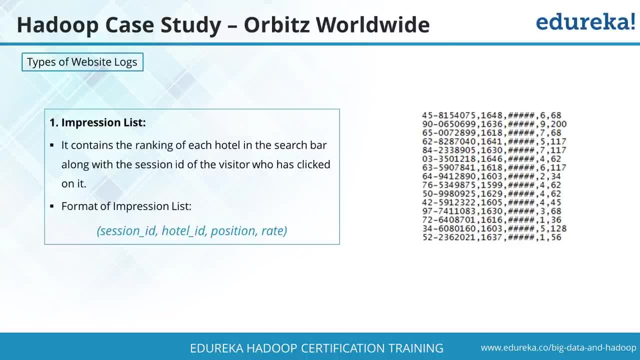 be at the third position there. what should be the position of each hotel? we should push definitely to think from a business perspective. it makes sense for whichever hotel is getting most click, Definitely I should show that hotel at my first photo. right, that should be my best position. 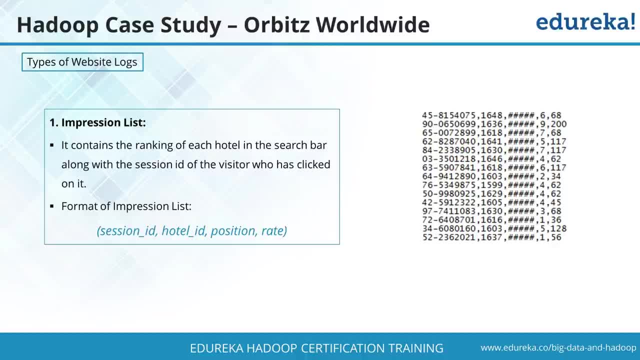 what I should give now. earlier that was not happening with them. they want to fix that problem. and second issue was: can you notice this? hash, hash, hash. they also want to remove all this hashes, because this was some bad data. remember I talked about veracity. this is the problem. 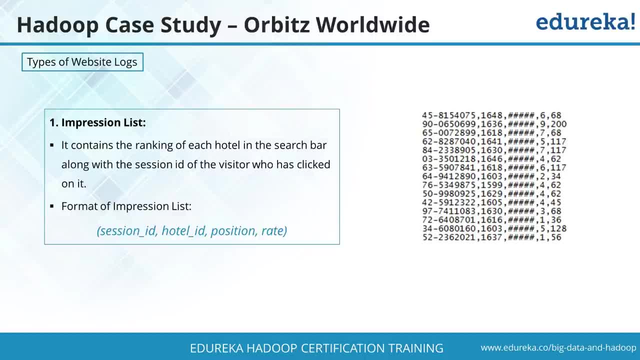 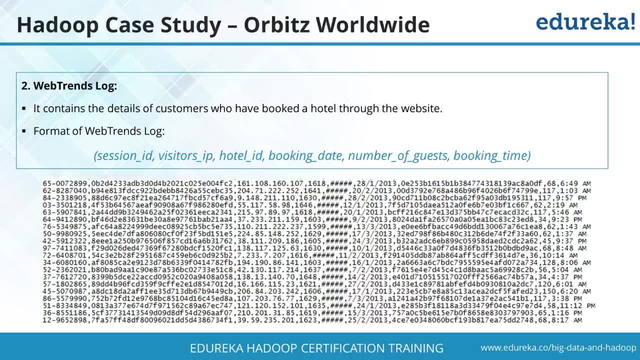 Now let's see what they have done. This is veracity now. similarly, they have one more data of different where they have session ID, visitor, IP portal ID, booking date, number of guests, booking time. all these details are there and here also they have the problem of bad data. 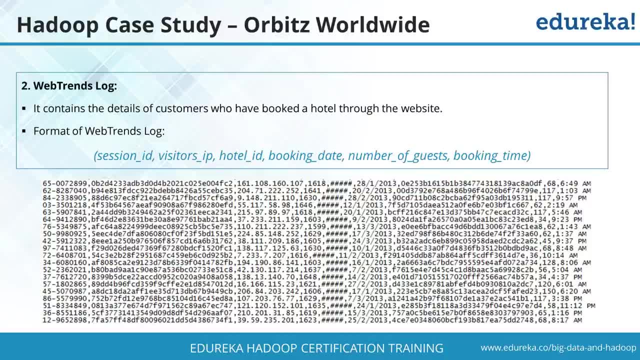 So they have to first fix it. so what they did as a first step was they have written a MAC reduce code. I'm not going to walk you through that MAC reduce code, because that will. you will not be able to get it if we have not already done this. 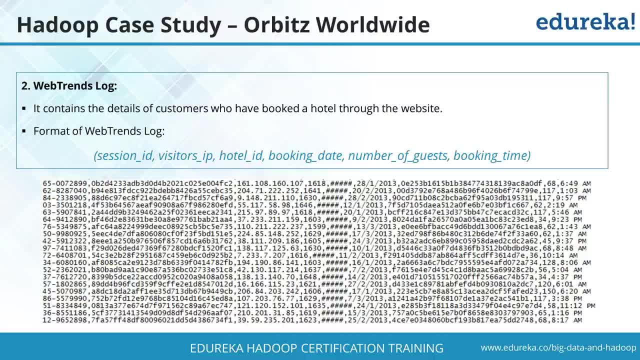 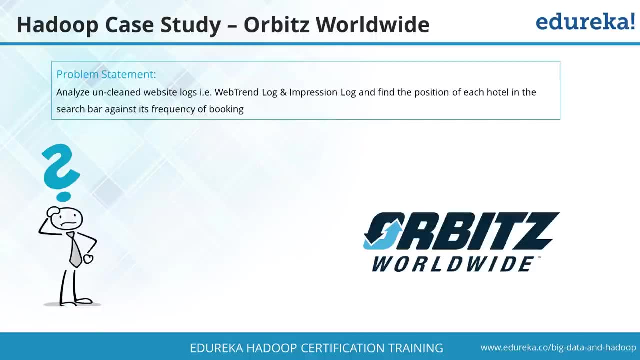 But they have written as effective MAC reduce code and using that, they were able to clean this data. okay, so using that, they were able to clean this data. Now, further down the line, now, once they have done all thatnek, now the major problem is how they can analyze everything and see that, whichever what should be the perfect position, 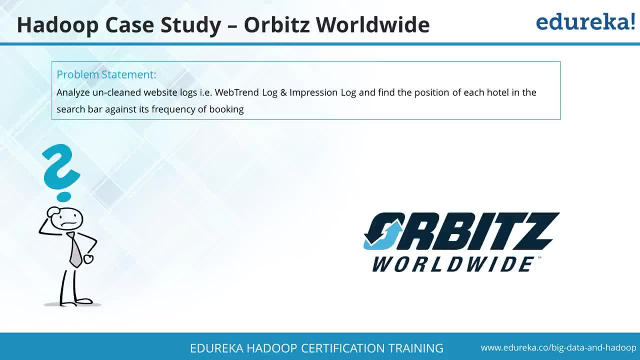 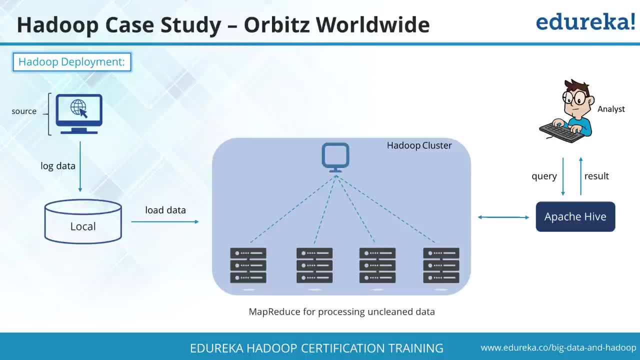 of each hotel. that is now my important path and that depends on the search bar against the frequency which hotel getting booked the maximum of those portions. Now, what they did? they first pull up the data, they put it in the local drive. they after that they brought it to the Hadoop cluster. 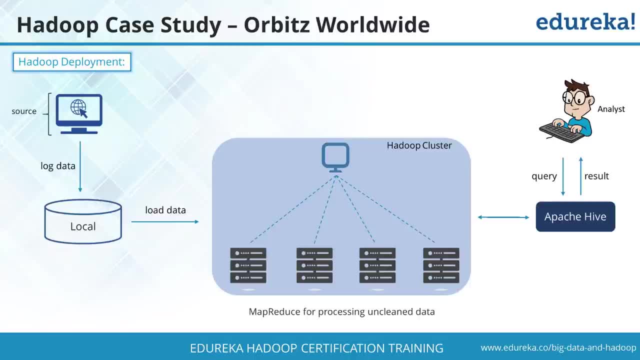 they clean the data, then, after cleaning, they put it into Apache Hive, because Hive is a SQL kind of tool where you can apply lot of analytics. all the analytics will be done from here, the query will be given by analyst and Apache Hive will be giving the result. 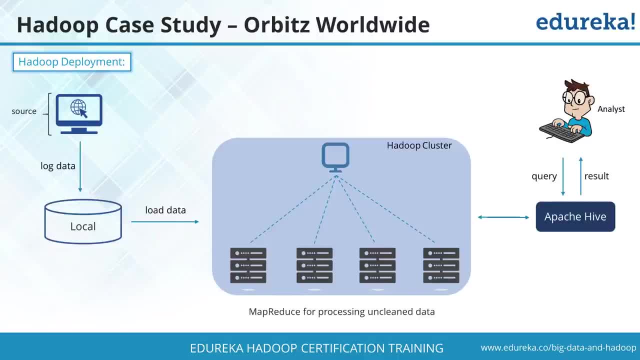 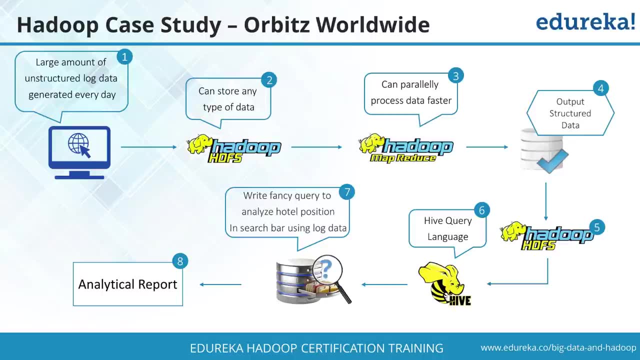 So this is the use case, what they were doing for that and to achieve that, what they did. they have large amount of unstructured log data. they store any kind of data like the structure, unstructured. they finally executed all the code with the help of MapReduce pack. 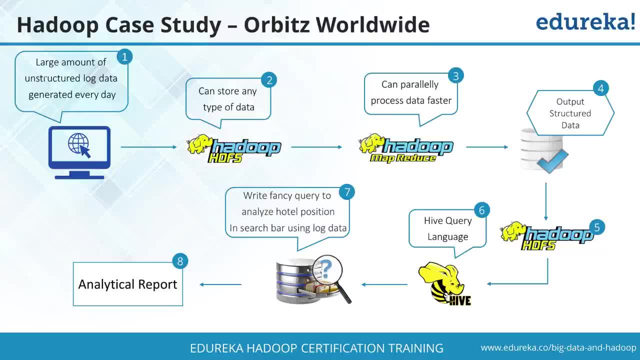 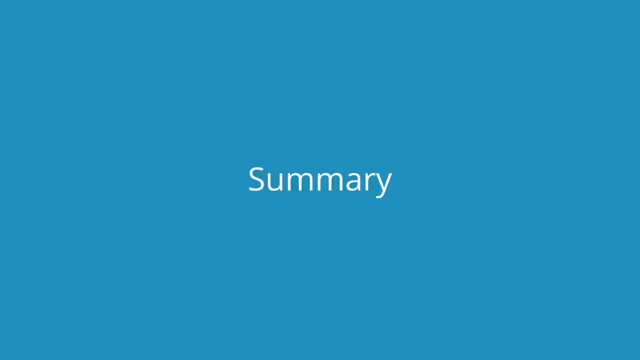 whatever output came out as a structured data, they spread it to the Hive, which uses HQL means Hive Query Language. then whatever output you are getting, based on that, they got the permission. then they just produce their analytical report. Let me just quickly go and show you this part in the machine. 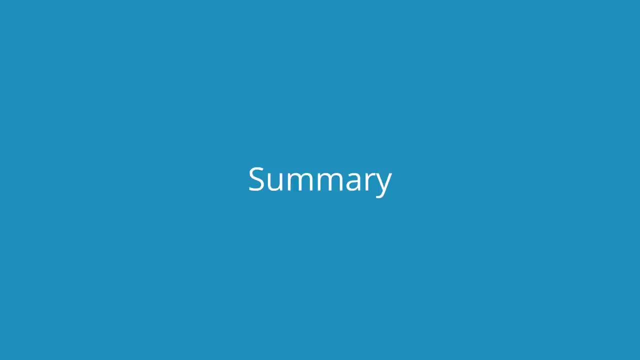 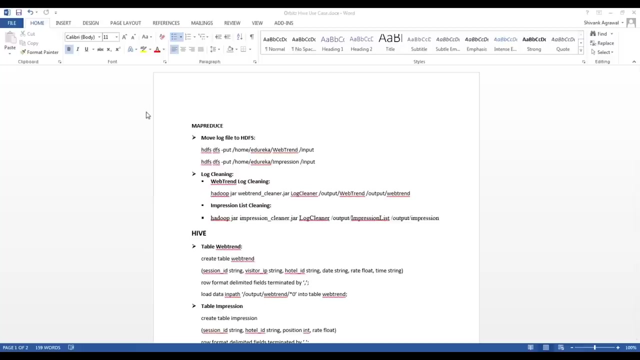 to give you a glimpse of how the output looks like. In fact, let me walk you through a document where we have all these things mentioned. Okay, look at this document. If you look at this document, what is happening here is we have our MapReduce code. 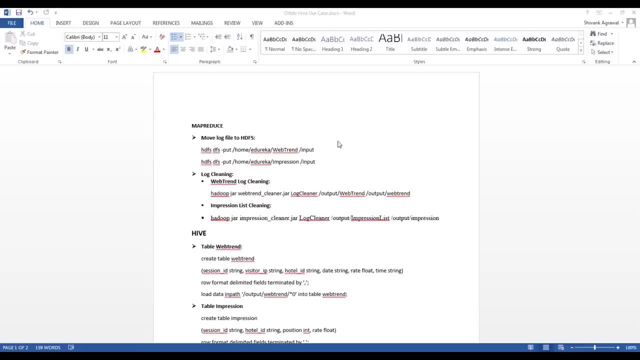 so we already have the MapReduce code We have. first of all, we are keeping all of our input files, what I just talked about, that we have the prints and impression. then we have created our MapReduce program. after that, we generated our jar file. Once we have done that, we are going to execute that jar. 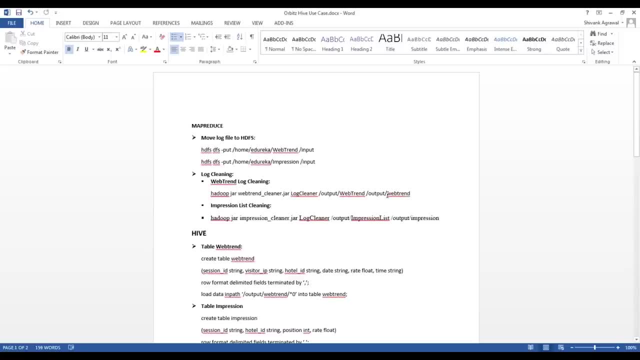 and in the output, we are going to have a cleaner data. This is going to happen for my impression as well as the print. Once that happens, I am going to get my structured data. Now I am going to get my structured data. I am going to go to my file. 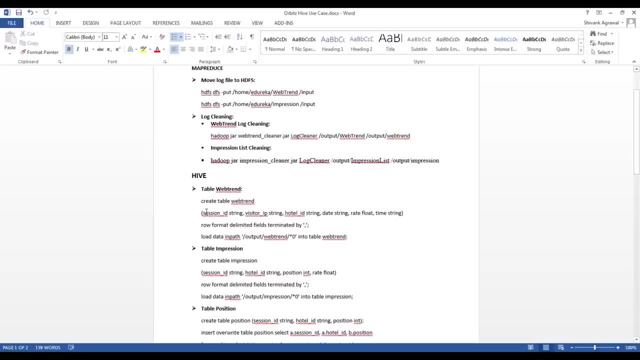 I am going to create a table web trend where I am going to create this table web trend having session ID, visitor IP and all. I'm going to show this in my VM as well. So this table will be created. After that impression table I have to also create. 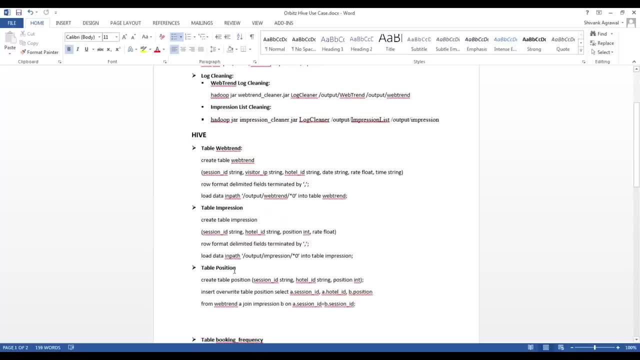 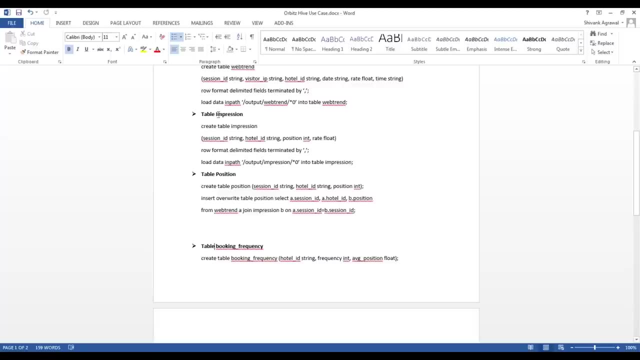 I'm going to load that clean data into these tables as well. Once this is done, we will create a new table called a position table, where we are again going to use our join with all these store tables And load our data and after that, once it is done, 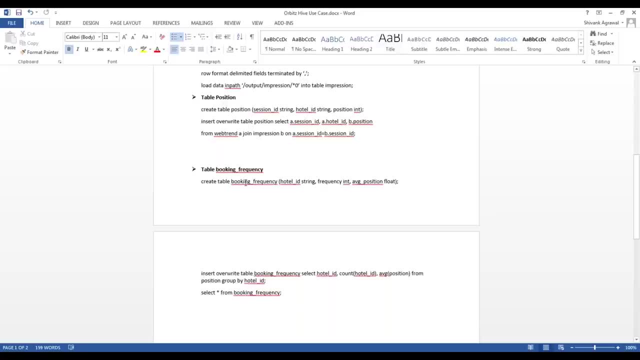 we will create a booking frequency table which is going. once I insert this data of position to it, I will be able to do the analysis. by doing this count How many number of times this hotel is getting listed, What is the average position it is making up. 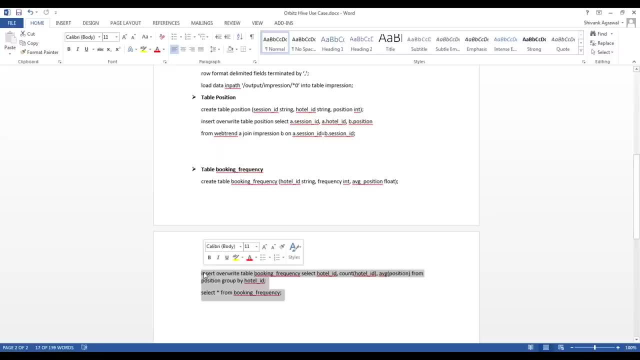 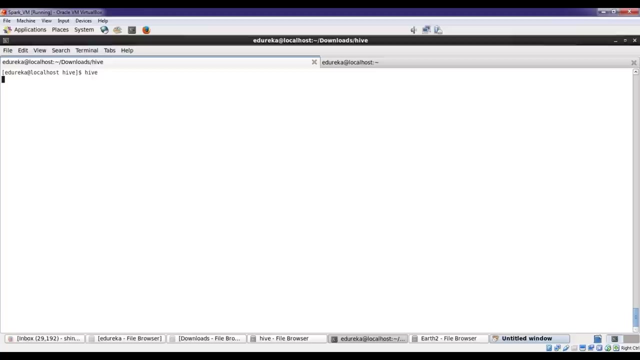 And this is how I will be able to tell that this is my. this should be my exact position, So let me show you quickly this booking frequency. That's how this looks like. In order to do that, let me just quickly get connected. Let me just quickly get connected to my hive. 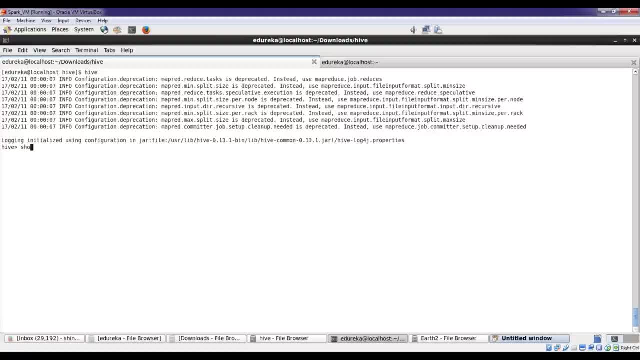 Once I am there, we can also list all the tables. So let's say, I say that, show tables, You can see this table, right, We have this impression, we have this position. we have so many tables available with us. Now, these tables are there. 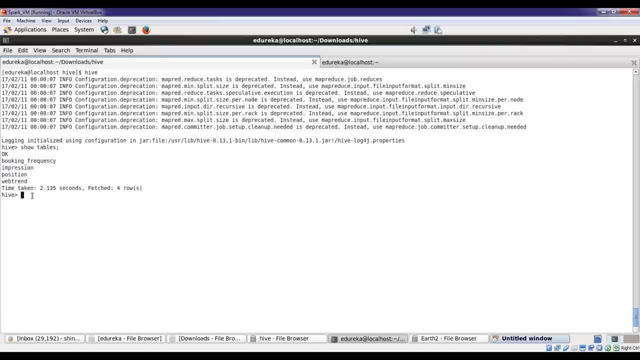 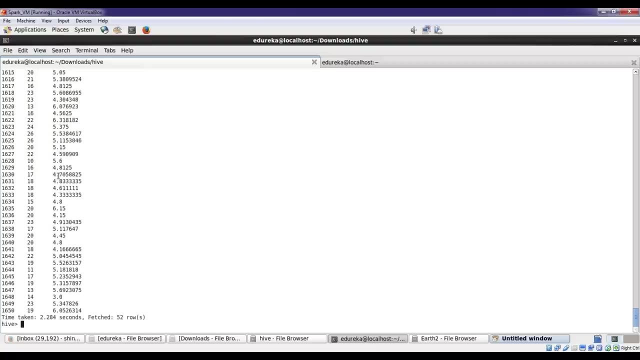 We want to look at the whole booking frequency for what we have seen. So let's see this: Select std from booking underscore frequency. Look at this output Now. this will show me the number of counts the hotel is being looked at, right. 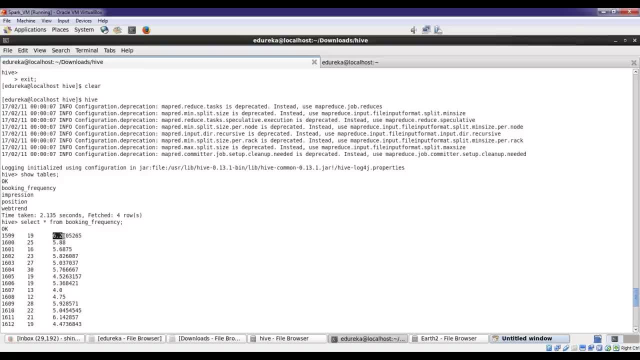 What was the number of times it is being done? and then can you see, the current position is this, but we want to push it at some other position now, right, So whichever is the most frequently being seen- or not, I will now with this analysis- will be shifting. 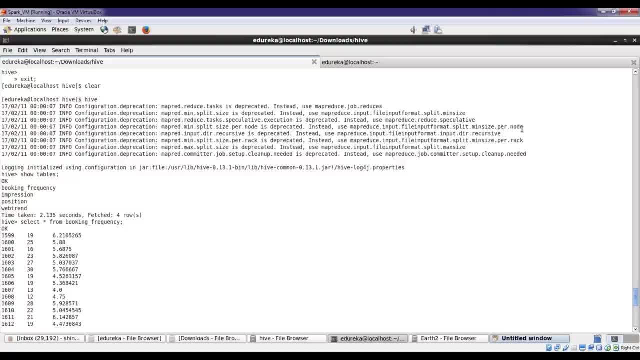 my positions accordingly. So this is how you will be performing your analytics. So let me go back. So this is how. this is just a very simple use case, what we have shown you here. Once we generally go through all these things in sessions. 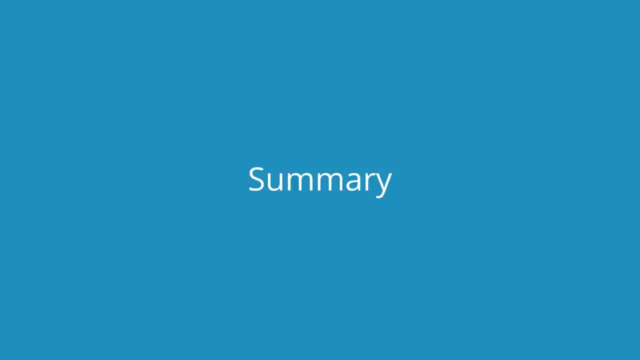 we walk through in detail about all these portions We walk through kind of. you will be knowing that, what are all the steps, What is involved here? properly, You will have all the details about that, because right now we cannot tell you about in this session. 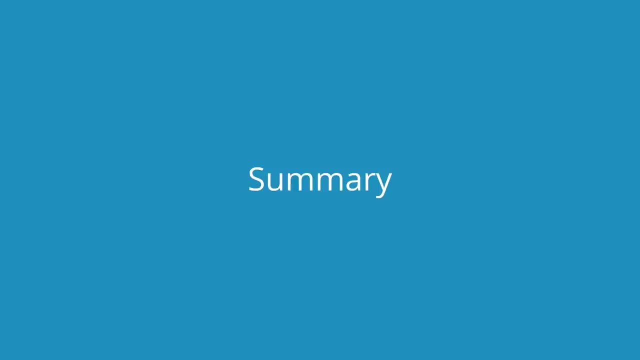 about how to write that map, this code, enough. but there you will be, learning each step by step and you will be able to easily do it on your own. To summarize everything Now we have all what is big data. we have understood that. where we discussed that big data is comprising: 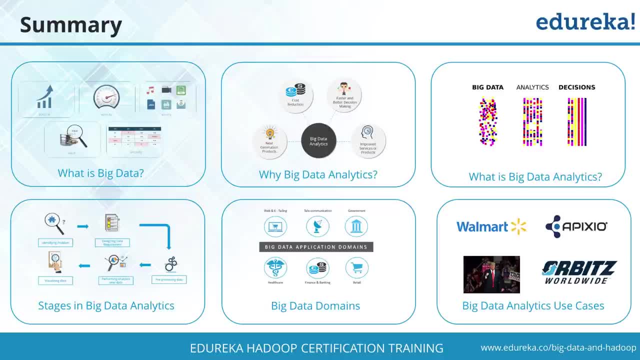 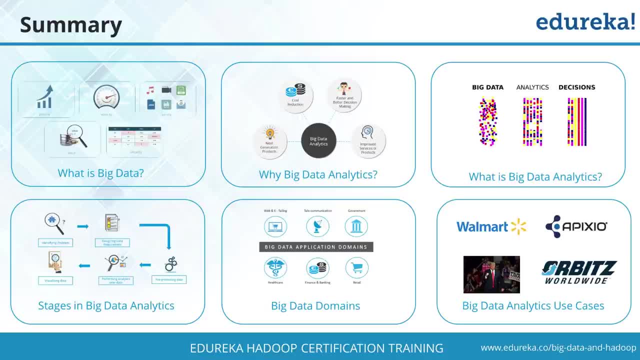 This is important part because it helps you to understand big data analytics. when you will be applying the analytics and then in the end you are doing the decision part, Then what are the stages you have in big data analytics? where you are identifying a problem, then you are doing the data requirements. 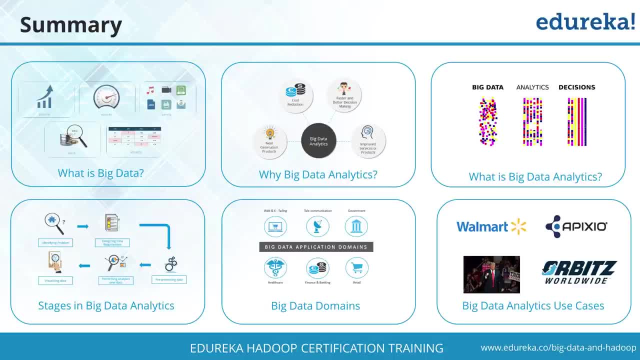 pre-processing of the data, applying your analysis and visualizing your data. What are the domains we do have? we have seen that these are very limited domains, what we discussed. there are many more which are possible. then how a person became a president of US by using this. 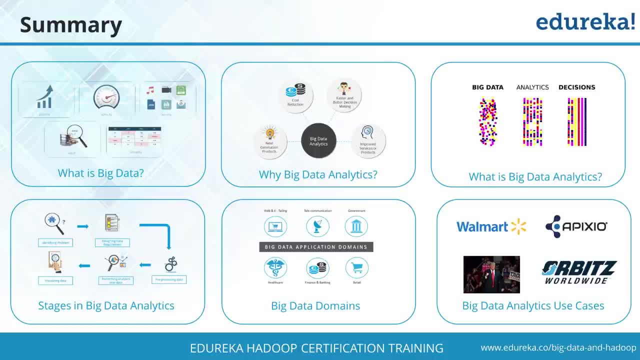 How a team can run a workup of people by using this. So all these examples also we have discussed in detail and these are the topics we have discussed. So I hope you have found this session useful. You are able to make out what exactly.